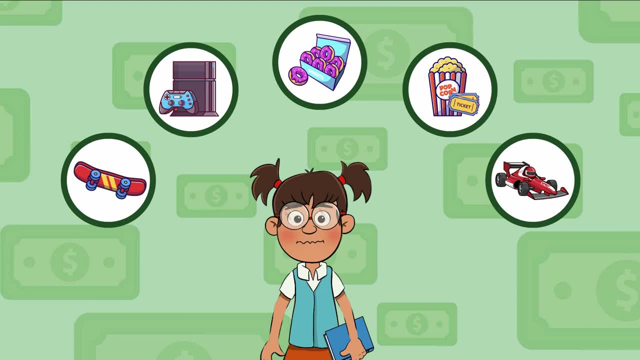 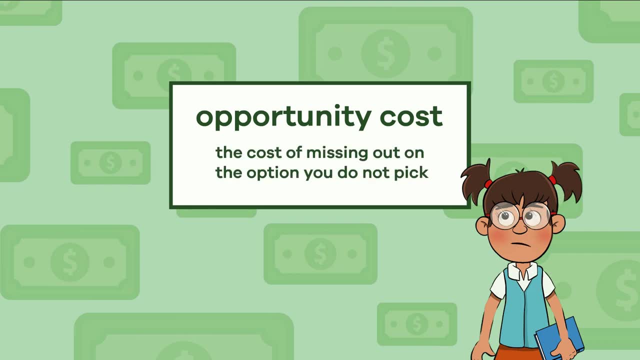 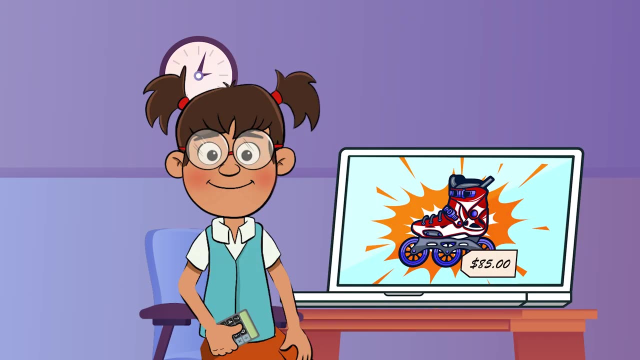 This is called an opportunity cost. An opportunity cost is the cost of missing something. An opportunity cost is the cost of missing something And missing out on the option you did not pick. Let's use Frankie as an example. Frankie wants to buy a new pair of rollerblades, which cost $85.. 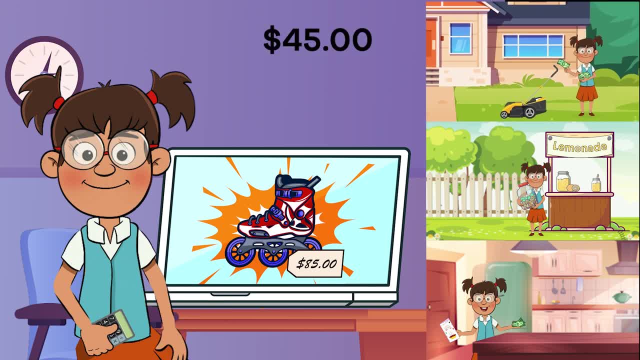 She has earned $45 from mowing her neighbor's lawn and running her own lemonade stand. Her grandmother gave her $20 for her birthday. She finds out that the rollerblades she wants will go on sale for $70.. She finds out that the rollerblades she wants will go on sale for $70. 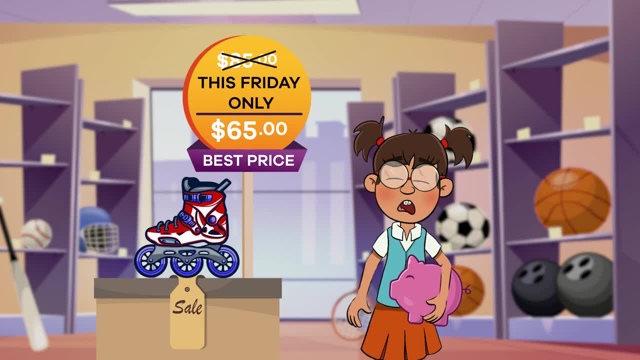 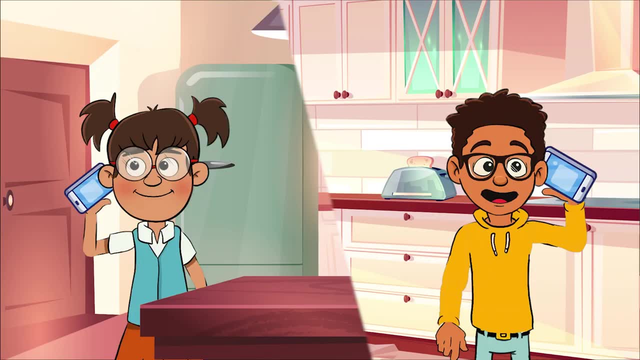 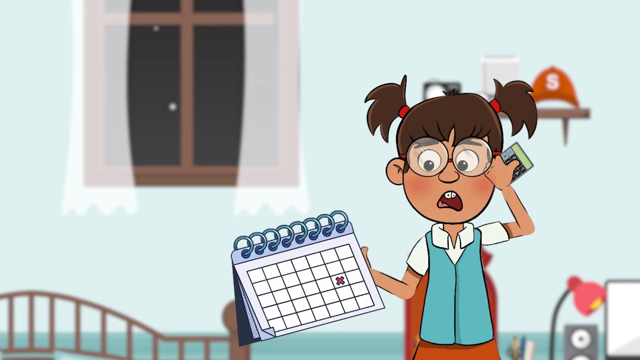 She finds out that the rollerblades she wants will go on sale for $65 for one day only- on Friday. Later that day, Frankie's best friend invites her to go see the latest superhero movie at the movie theater With some friends. on the same Friday the rollerblades will be on sale. 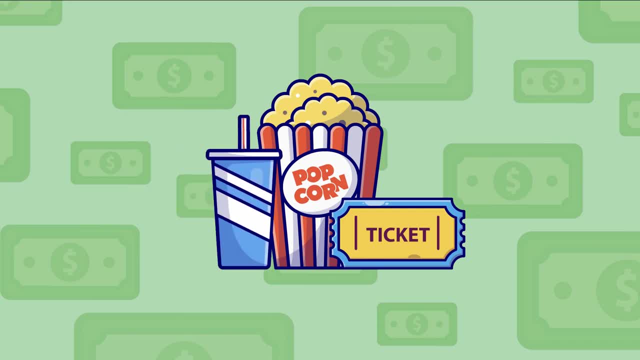 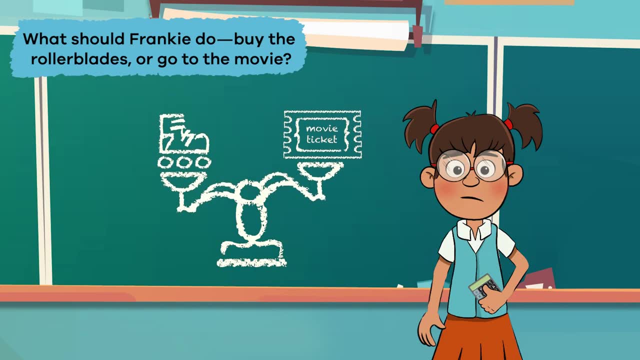 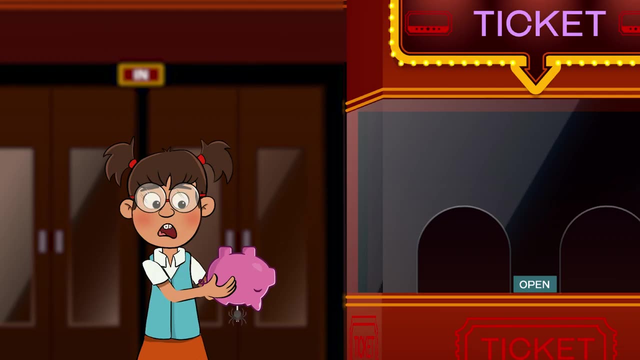 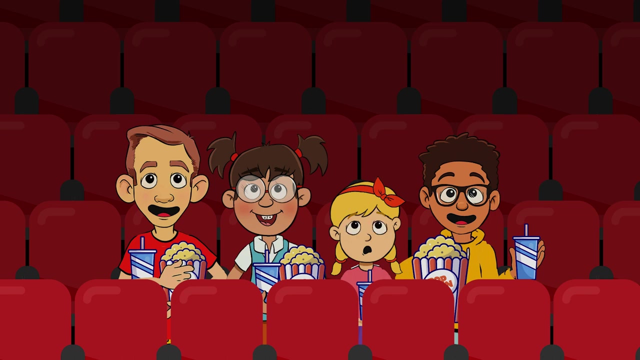 The movie, popcorn and soda will cost around $20.. What should Frankie do? Buy the rollerblades or go to the movie? If she chooses the rollerblades, she won't have enough for the movie with her friends. On the other hand, if she chooses to go to the movie, her opportunity cost is the rollerblades not being on sale anymore. 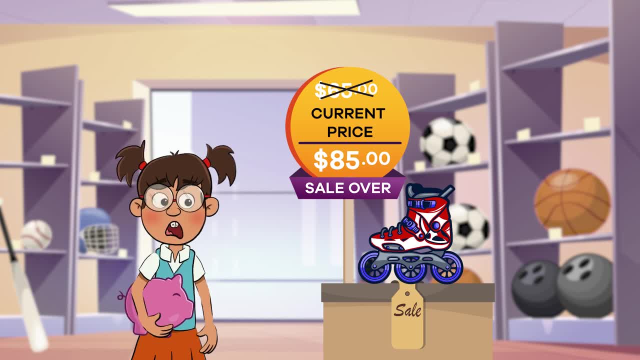 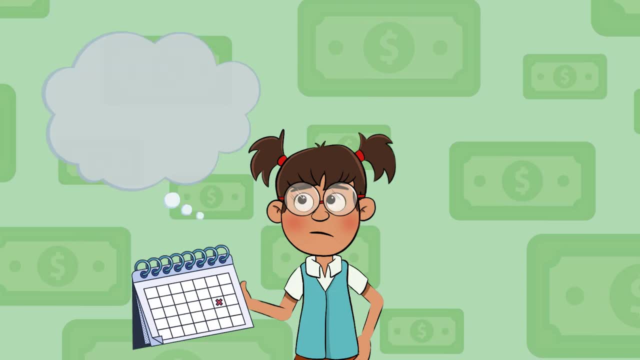 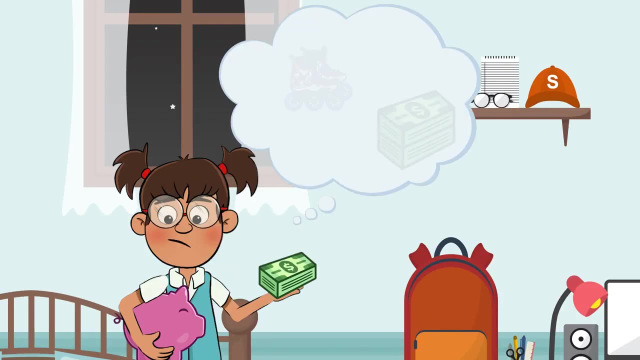 which means she will not have enough money to buy them. Hmm, Frankie must decide what works best for her: buying the rollerblades on sale or the movie with her friends. She also must decide if she wants to spend all $65 of her saved money or just part of it. 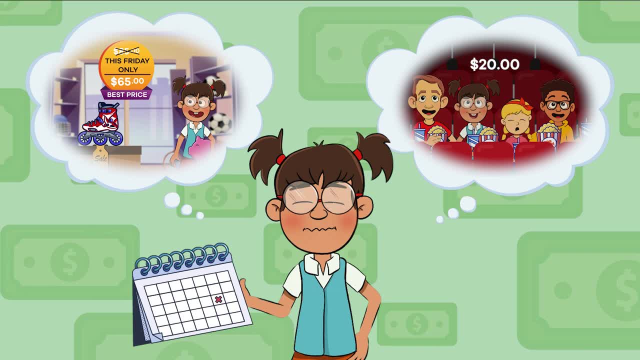 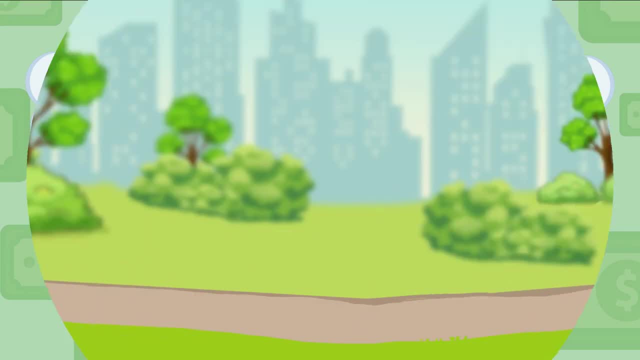 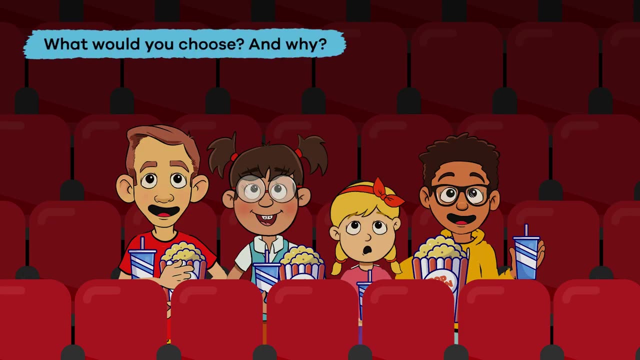 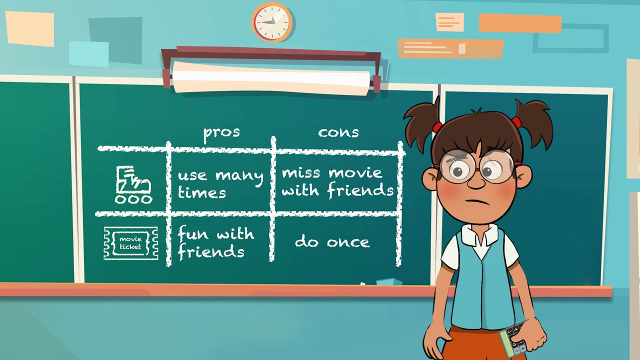 These decisions are personal and the consequences are not life-threatening. It's about choosing which you value the most. when you decide Rollerblades or friends, What would you choose and why? The next time you are deciding between two or more costs, try making a list of pros and cons and go from there. 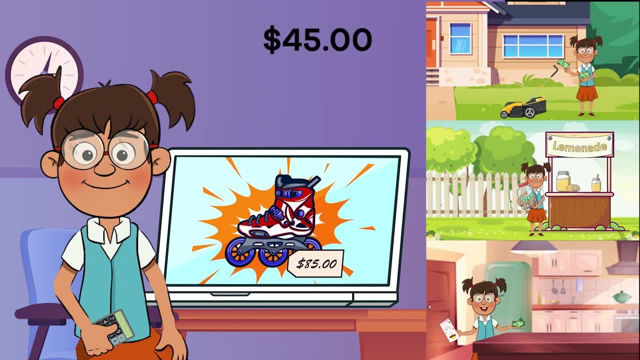 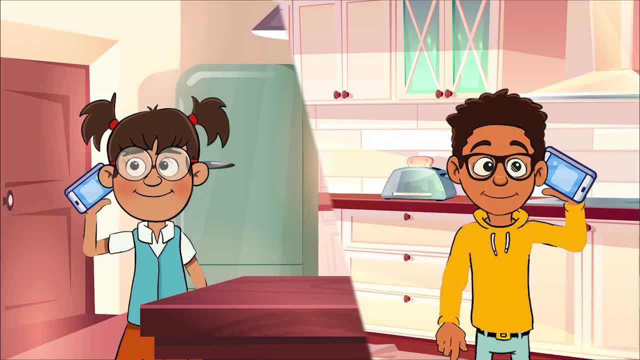 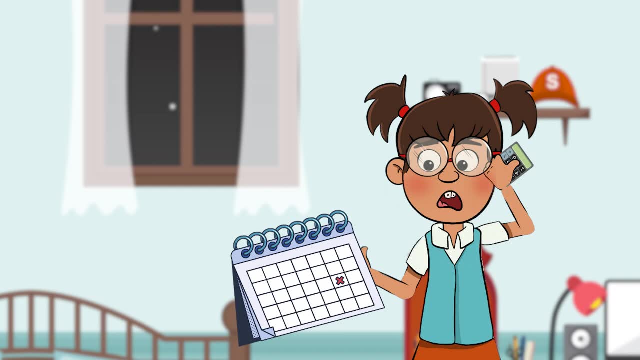 She finds out that the rollerblades she wants will go on sale for $65 for one day only: on Friday. That day, Frankie's best friend invites her to go see the latest superhero movie at the movie theater with some friends. On the same Friday, the rollerblades will be on sale. 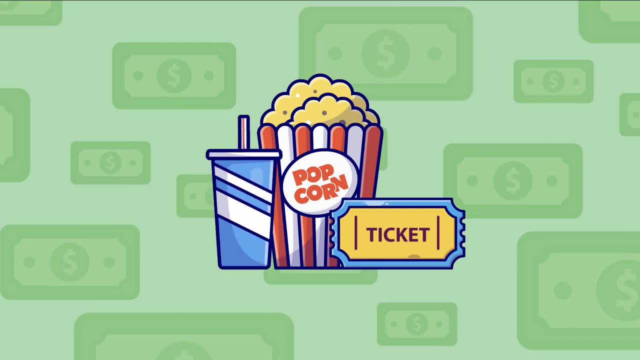 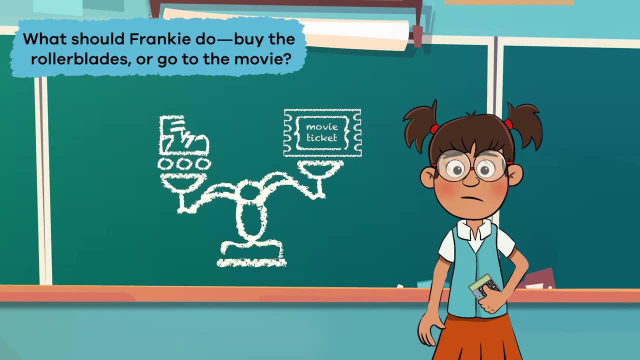 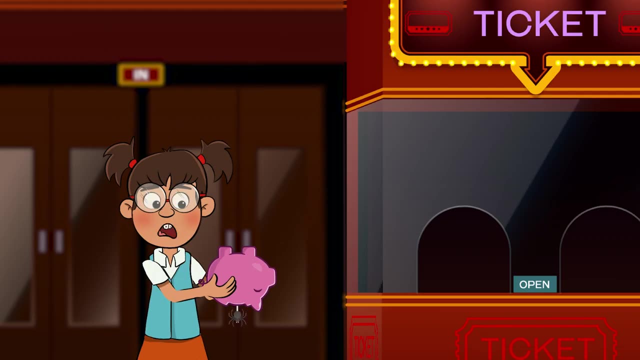 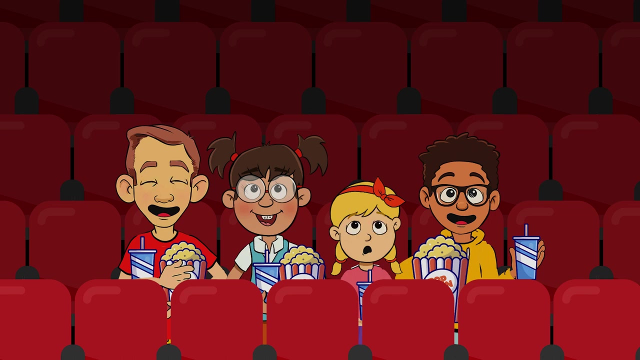 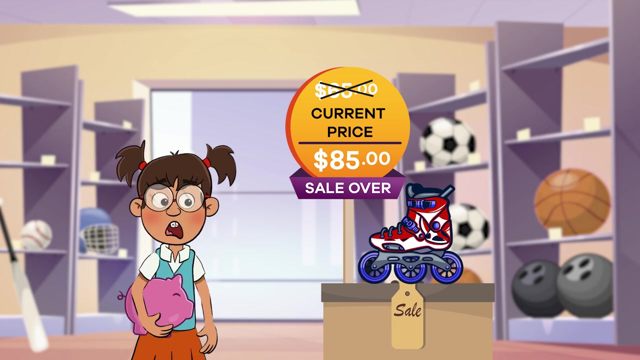 The movie, popcorn and soda will cost around $20.. What should Frankie do? Buy the rollerblades or go to the movie? If she chooses the rollerblades, she won't have enough for the movie with her friends. On the other hand, if she chooses to go to the movie, her opportunity cost is the rollerblades not being on sale anymore, which means she will not have enough money to buy them. 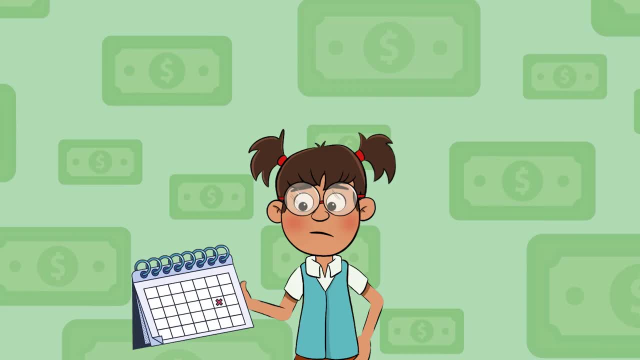 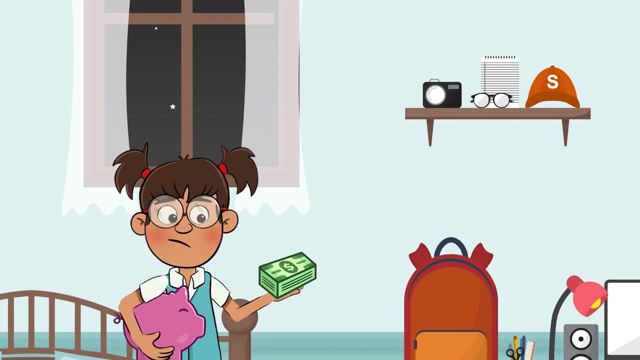 Hmm, Frankie must decide what works best for her: Buying the rollerblades on sale or the movie. She also must decide if she wants to spend all $65 of her saved money or just part of it. These decisions are personal and the consequences are not life-threatening. 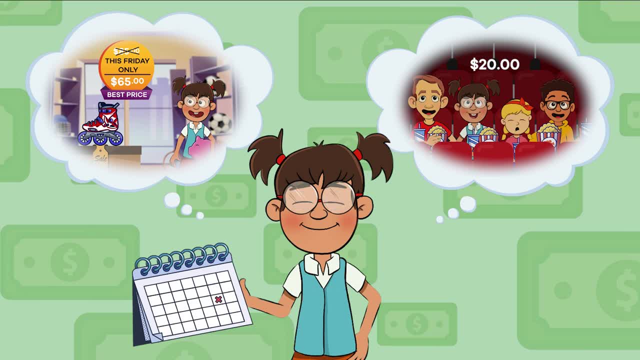 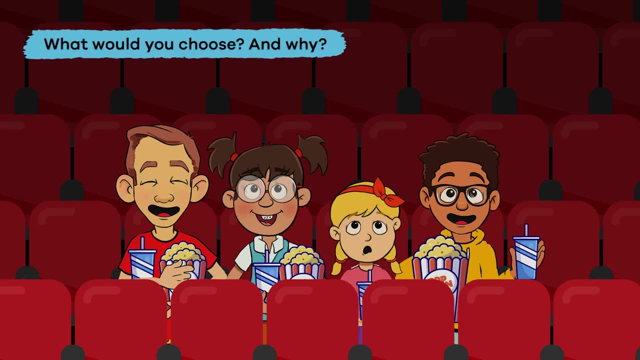 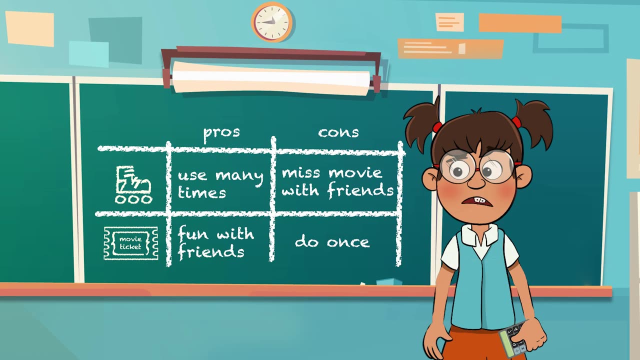 It's about choosing which you value the most. when you decide- Rollerblades or friends, What would you choose and why? The next time you are deciding between two or more costs, try making a list of pros and cons and go from there.